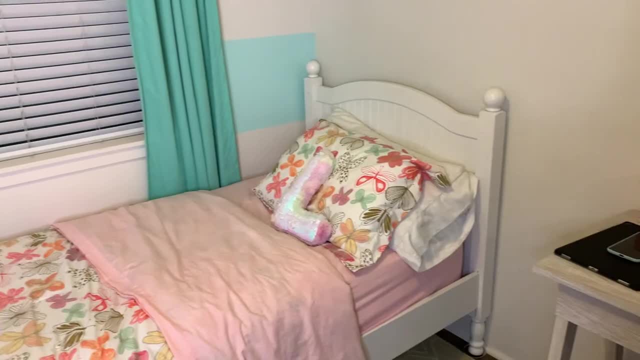 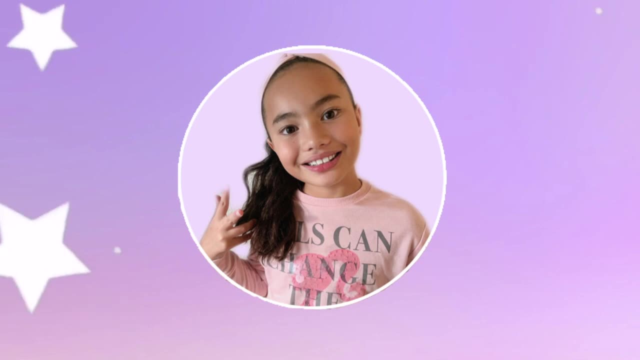 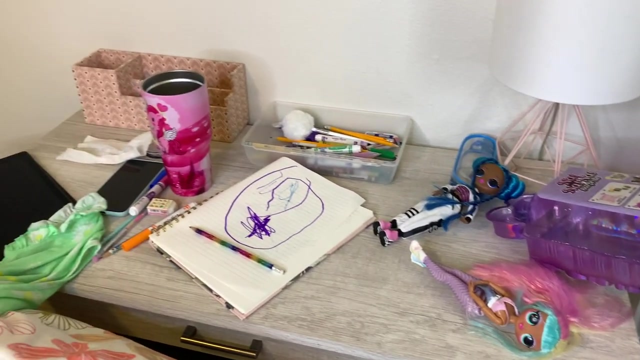 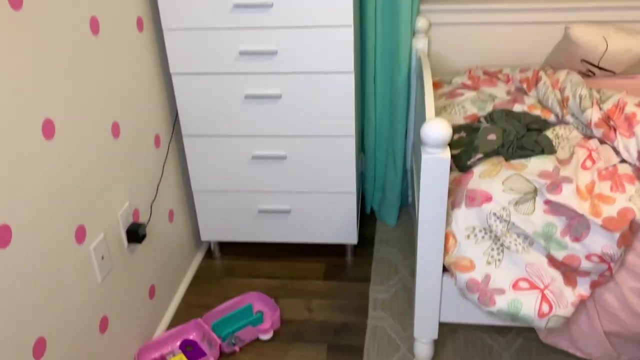 Watch me take my room from this to this. So this is my messy room. It's kind of embarrassing, but we're gonna get started cleaning it right now. First, I'm going to take all my laundry and throw it in the laundry basket. 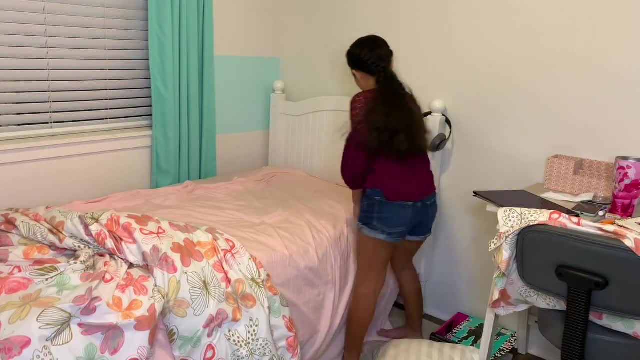 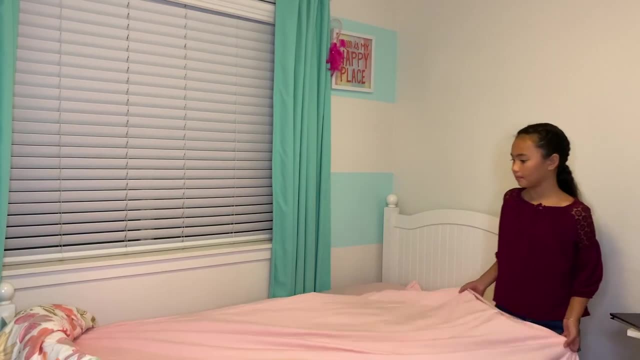 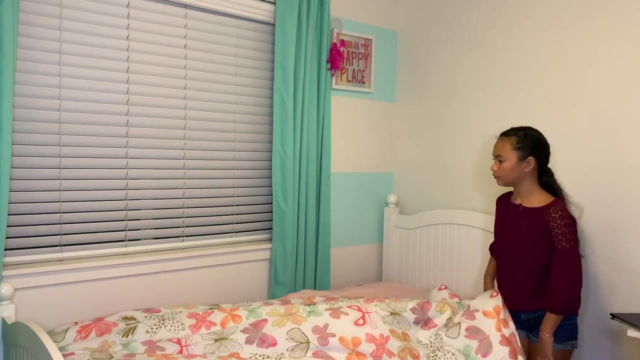 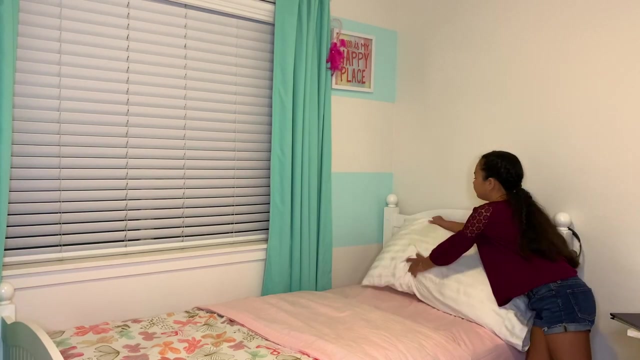 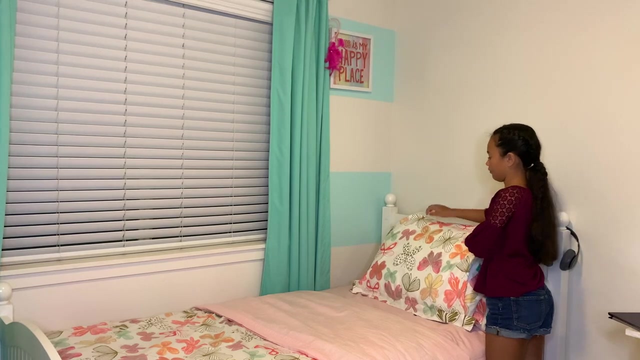 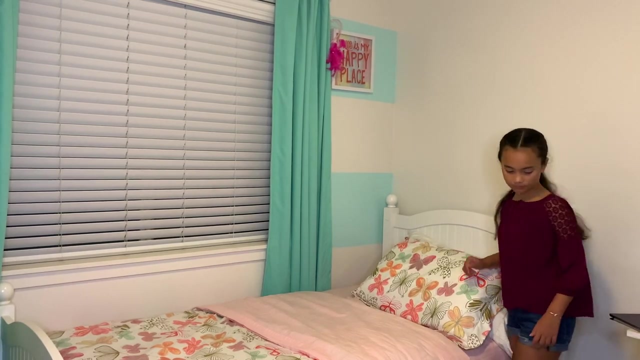 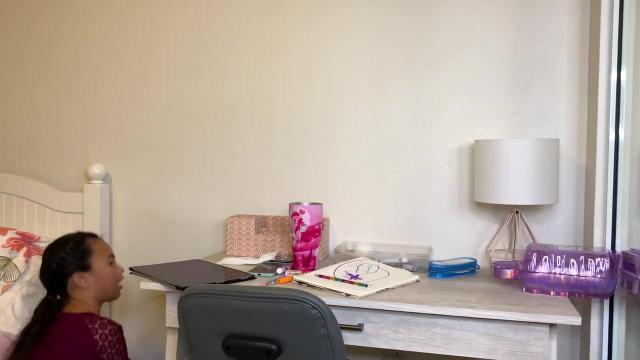 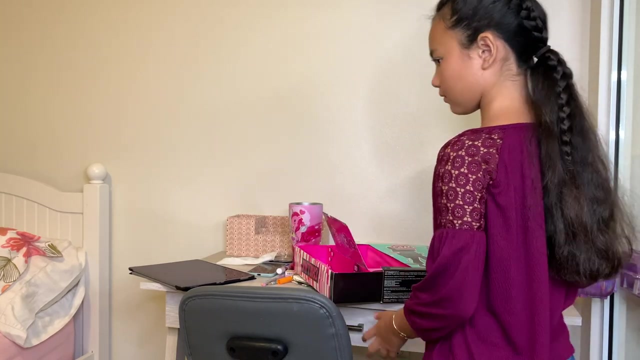 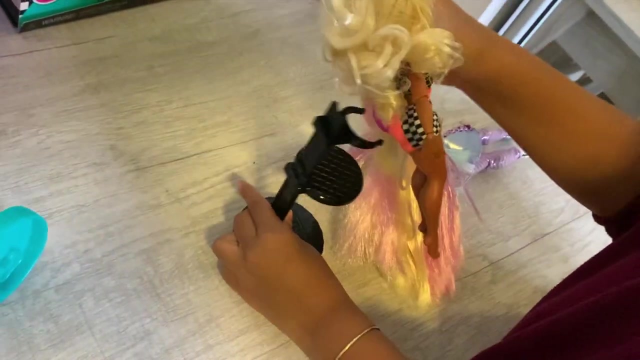 Then I'm going to fix my bed. I like to take everything off first. This part took forever, so I cut a lot of it out. All done Now. my bed is all nice and pretty. Now I'm just cleaning up my own J-Dolls. I'm putting Chillax in her box. 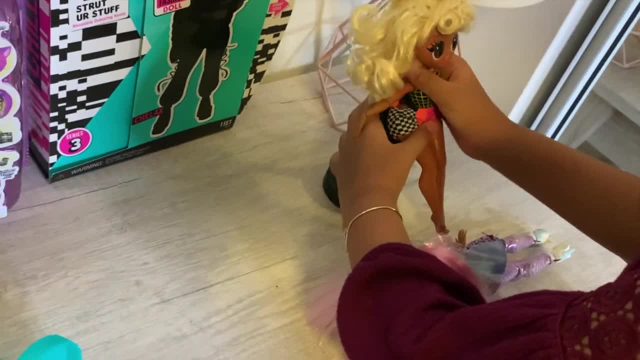 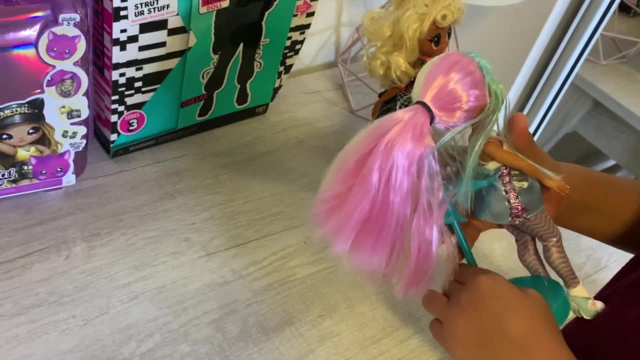 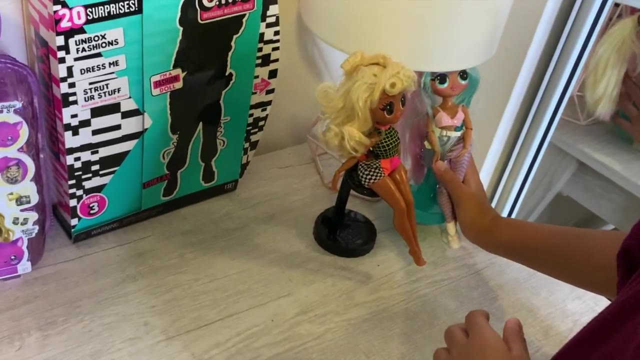 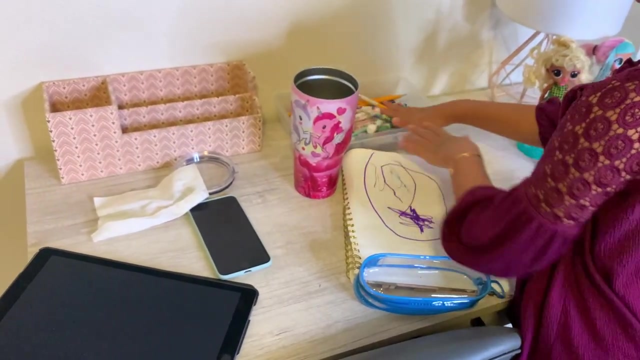 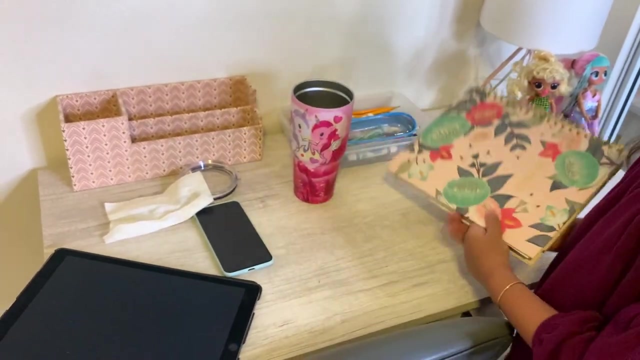 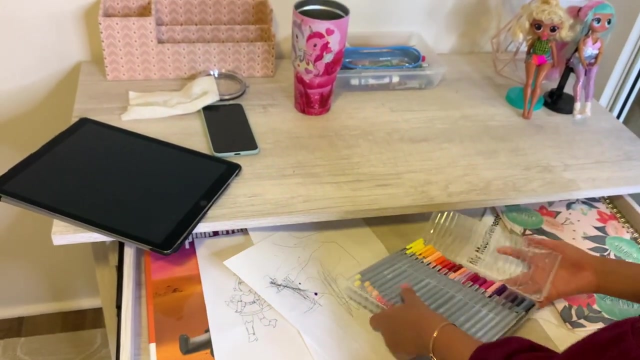 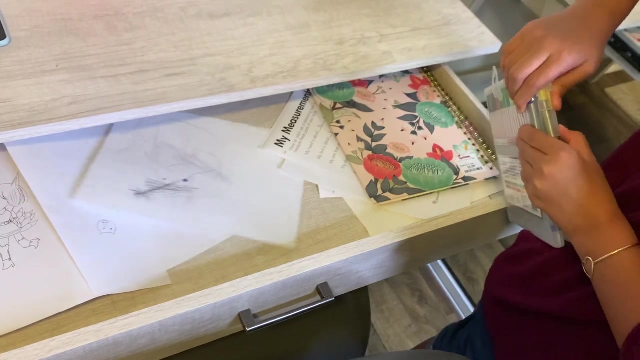 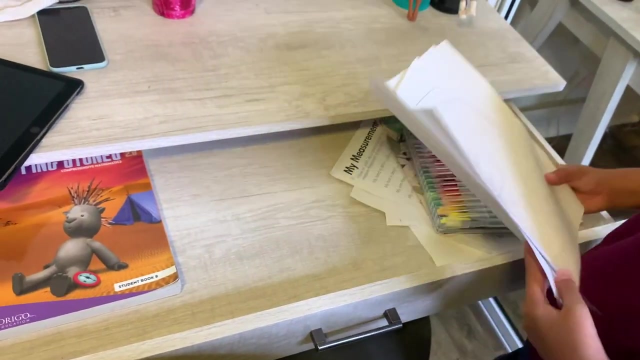 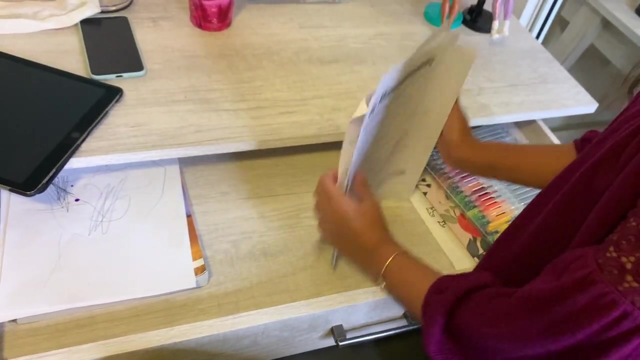 and I'm putting Speed's Jordan Candylicious on their stands. I'm just straightening up my desk right now and putting everything away. FYI, that's Malia's artwork. This drawer is really messy and I probably should have thrown some of these papers away. 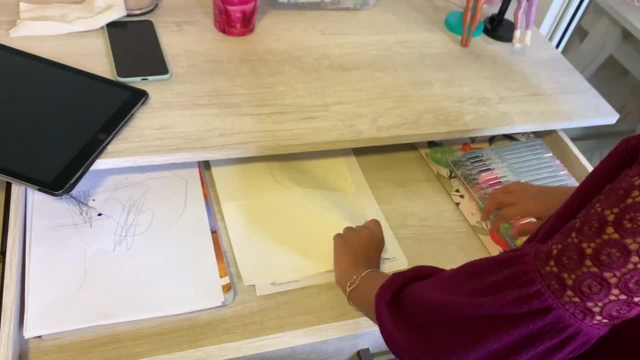 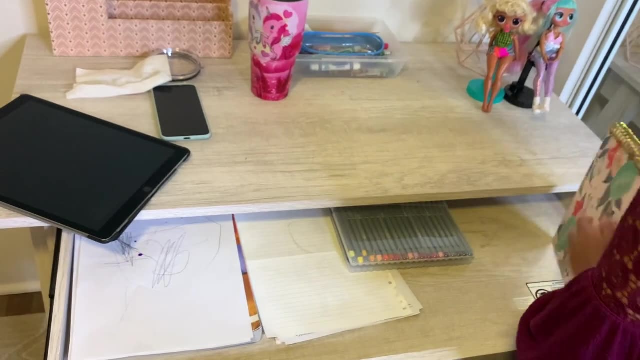 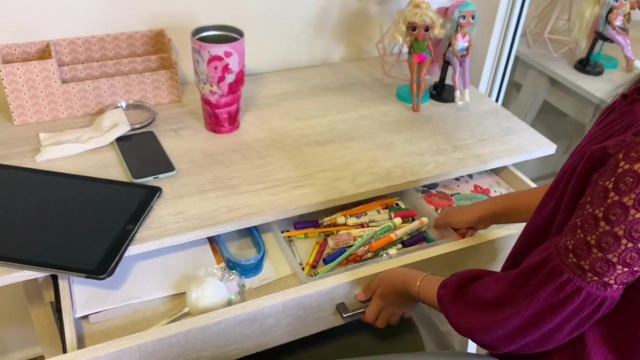 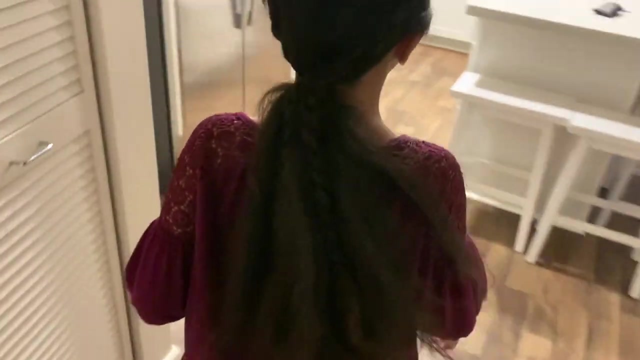 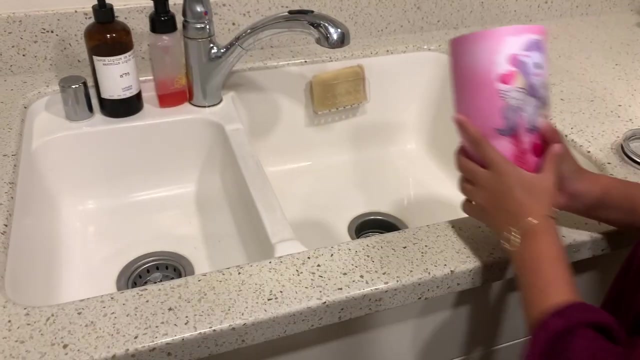 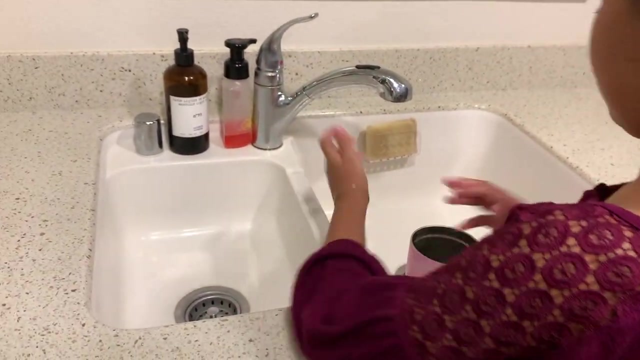 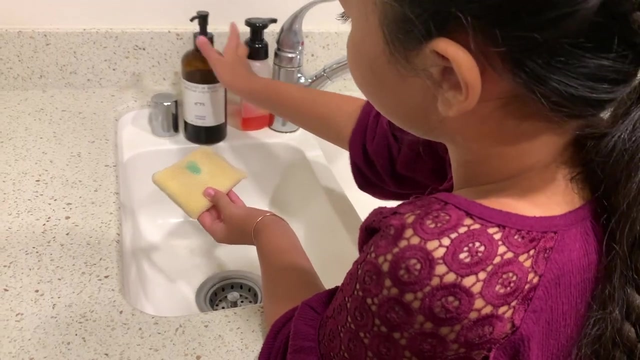 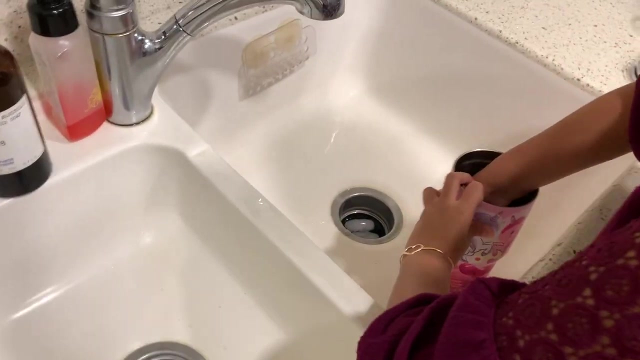 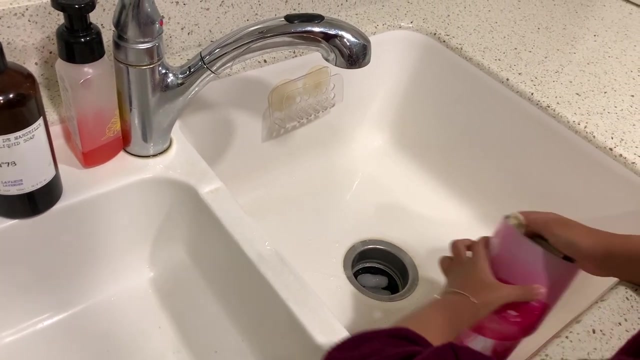 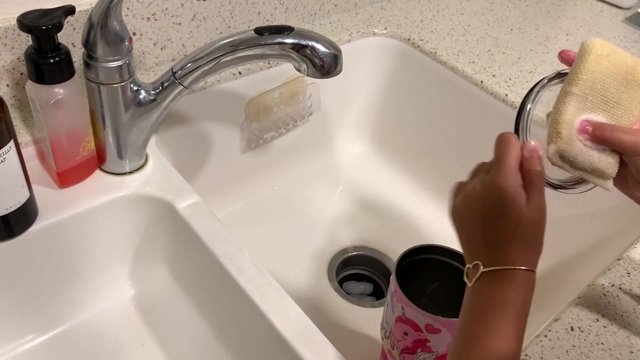 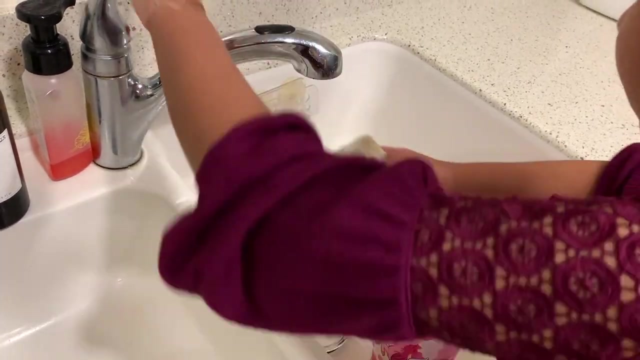 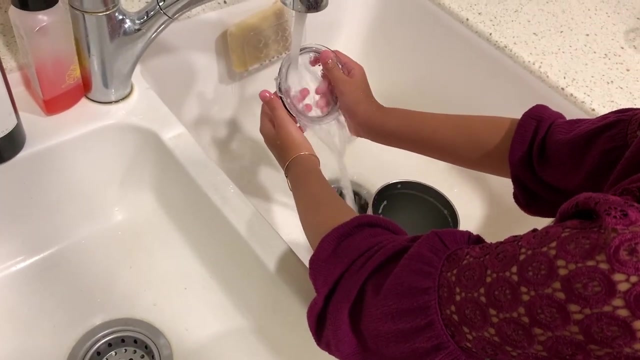 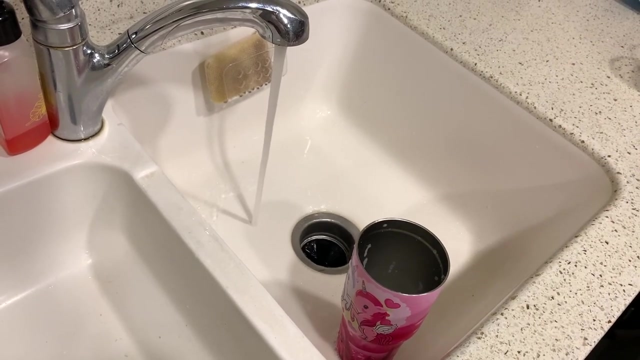 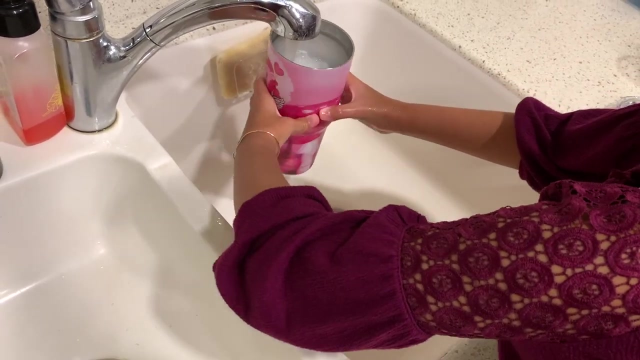 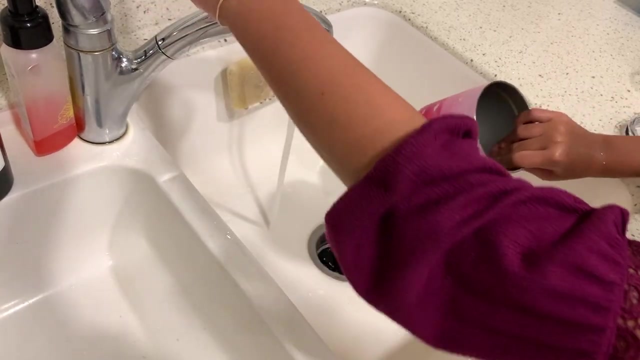 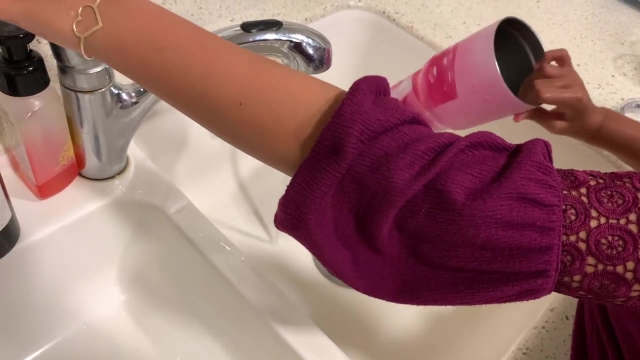 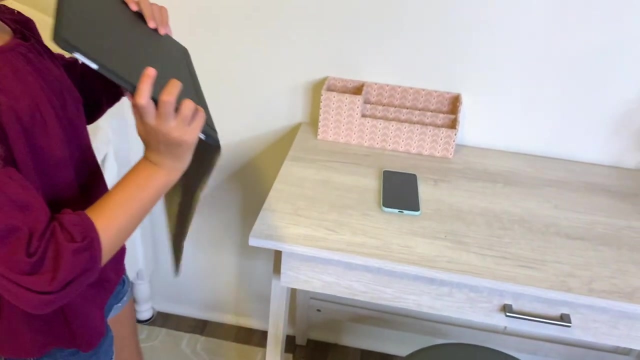 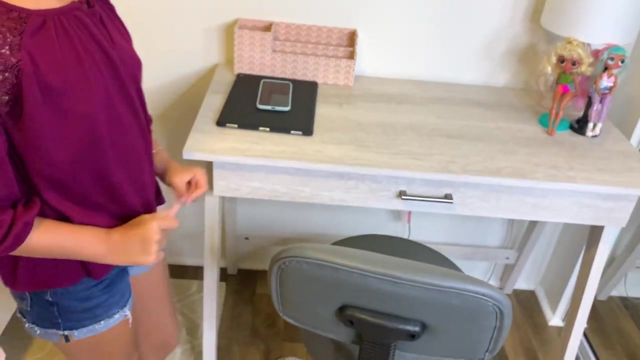 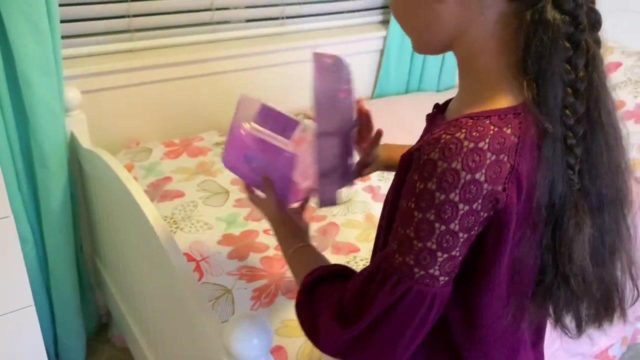 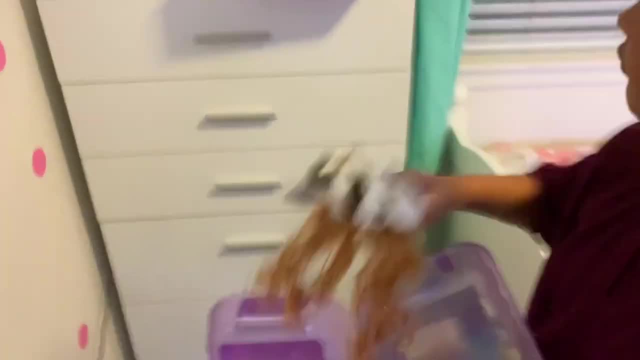 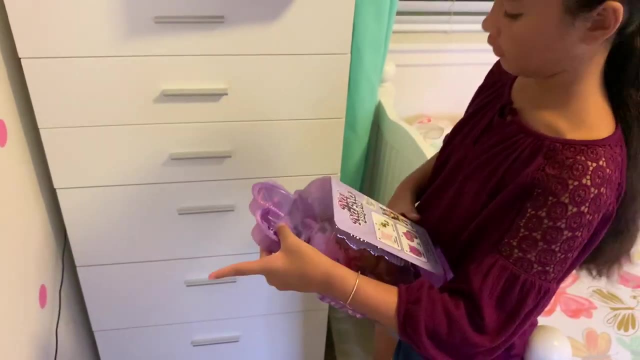 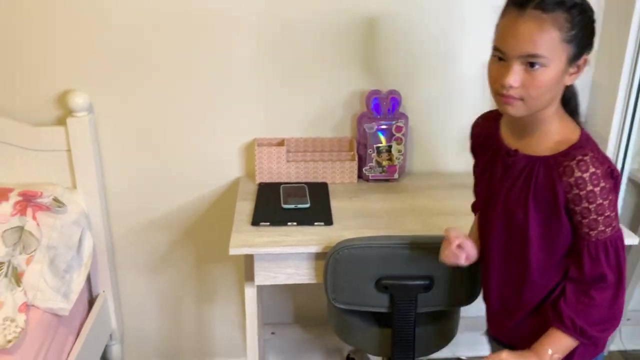 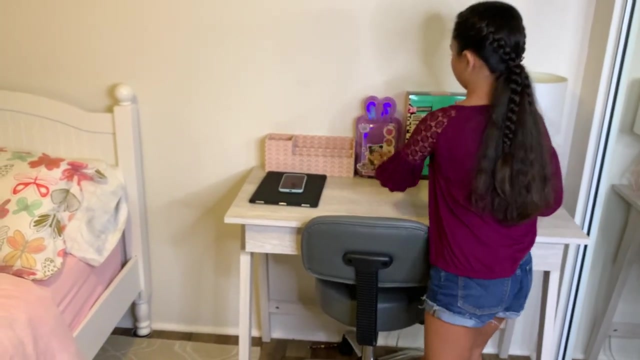 Sometimes I wash the dishes and load the dishwasher to help my mom. This is my Na Na Na surprise doll that I got from my grandma. She's super cute. I like to put my new dolls on my desk. I like to put my new dolls on my desk.